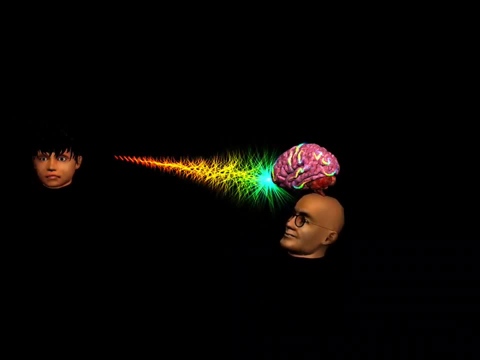 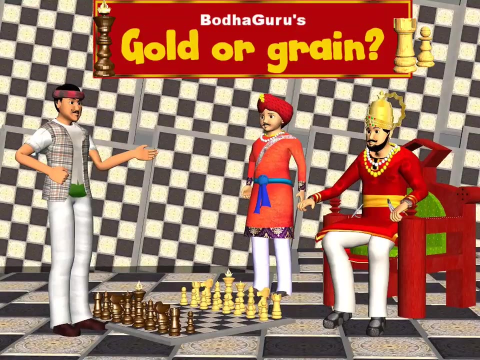 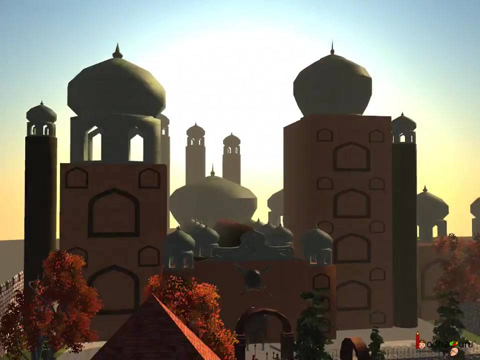 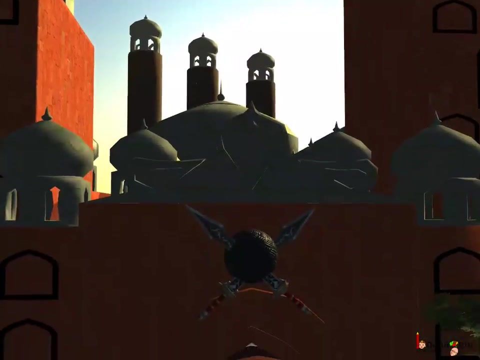 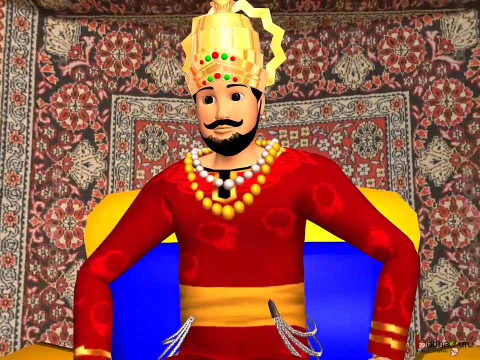 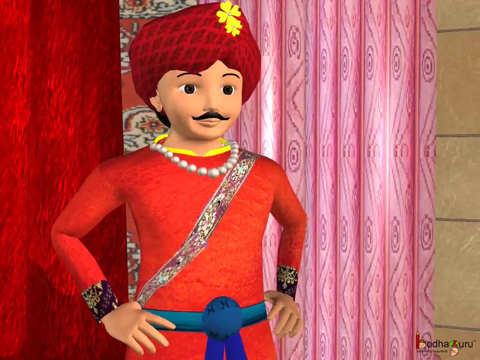 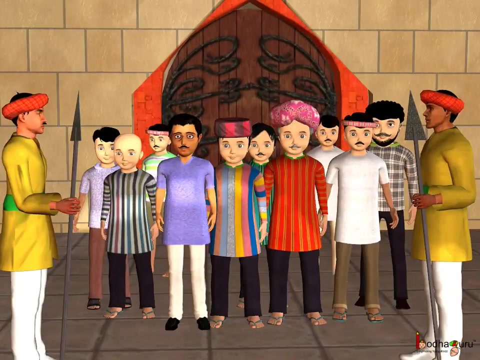 Once upon a time there lived a king named Veer Pratap Singh. He had a vice prime minister named Gyan Dev. The king liked to play indoor games, So he asked his people whoever will create the most interesting and challenging game. 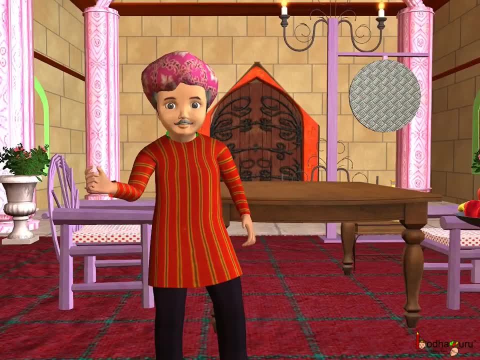 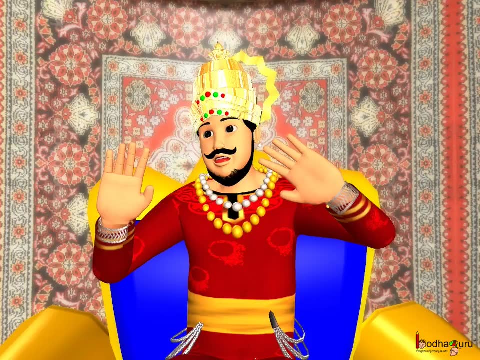 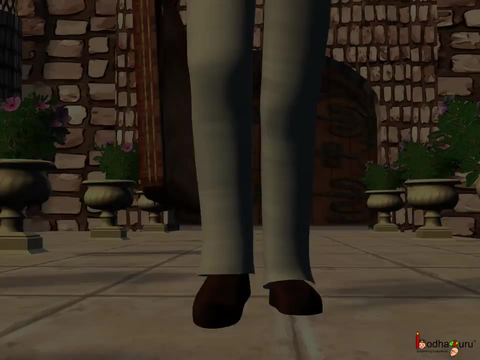 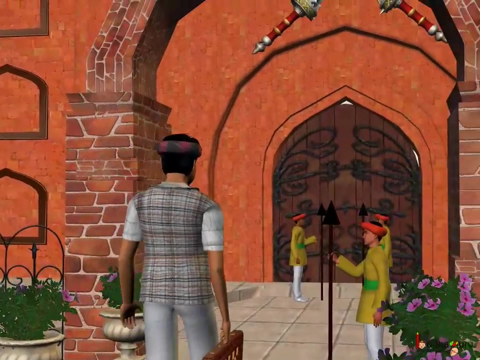 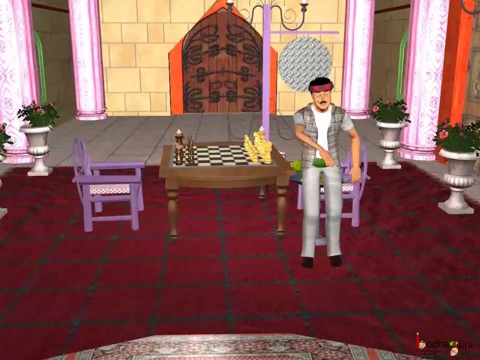 would be suitably rewarded. Many people came up with new ideas and games, but the king didn't like any game. Some were boring, while others were too complex to understand. One day, a man came and showed the king a new game called chess. 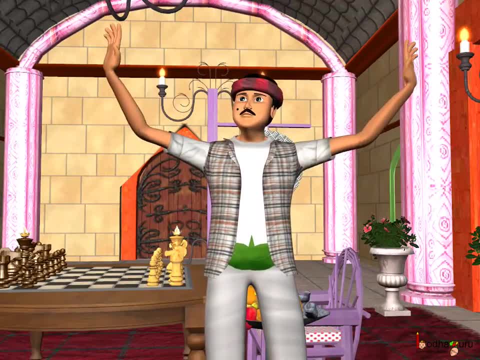 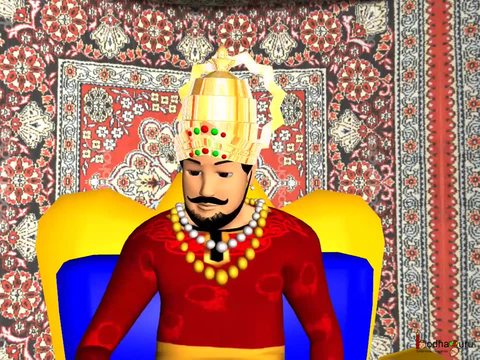 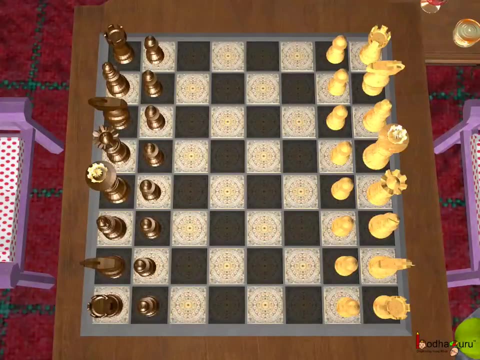 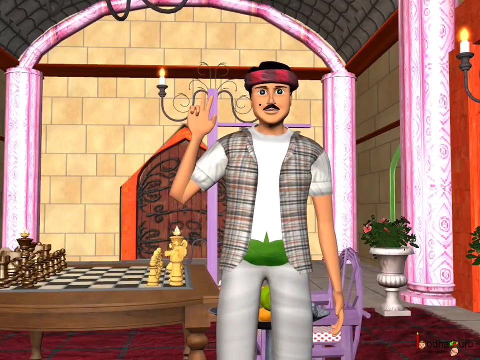 Your majesty, I have invented a new game. It is called as chess. Tell me more about it. This is a board game with 32 white and 32 black squares. The game is played between two individuals. Let's play, then. 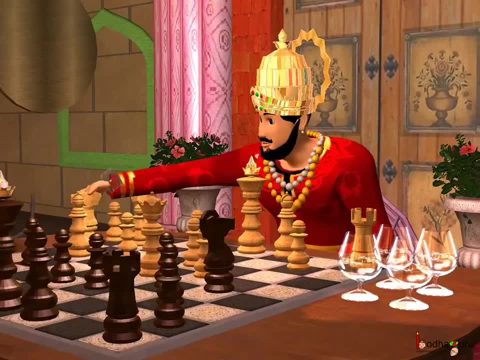 Let's see how it. it's how it's going to turn out. You are not intelligent enough, so you don't have to listen properly. Go for it. go for it First of all. actually, this game should come out to these countries 2 times. 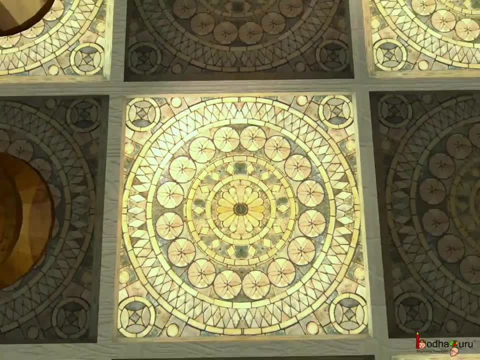 I, A ether, will name this Valley of Demons as my last name. I know all the facts and I really know why Your queens always exist. however, it doesn't matter whom I name, If the one who wins wins the game. 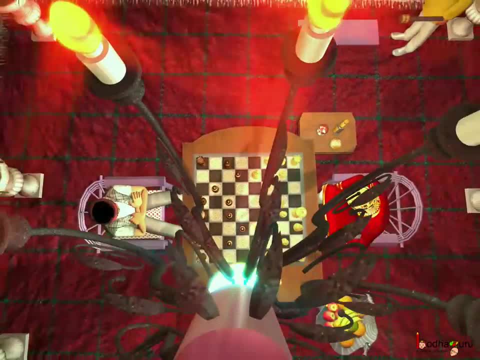 then I will take the word you have got to and move this in place with you, Because I have no part in it anyway. Now you see what happens. if you do that, Speak in different languages. If you do it, you will be the same people. 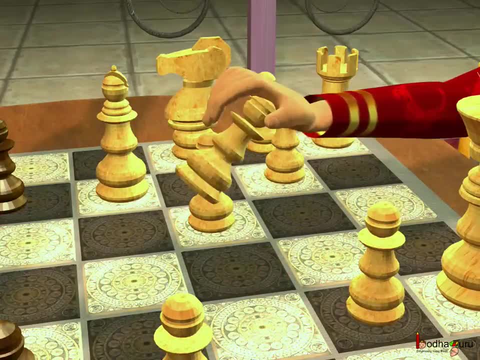 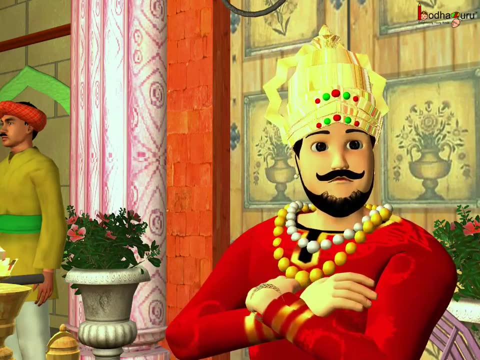 If you do get hurt, you will never be treated. this time. No, I am the king. You are like your club man. This is really interesting, isn't it Gyandevji? Yes, my lord, I can clearly see. 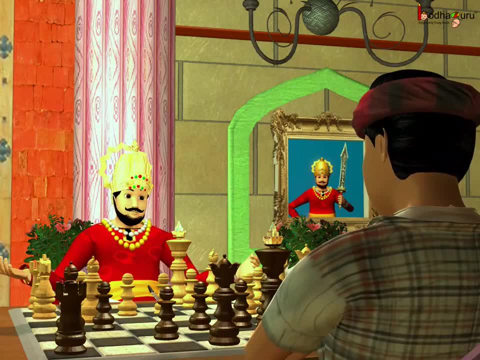 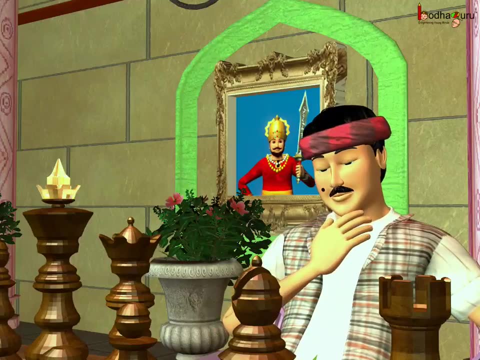 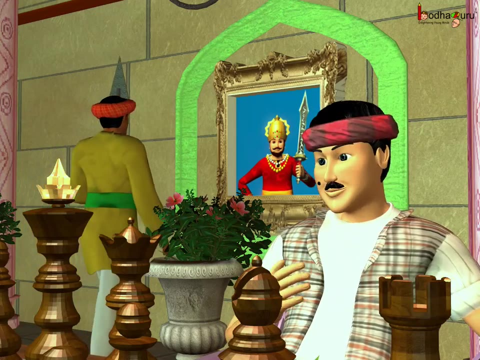 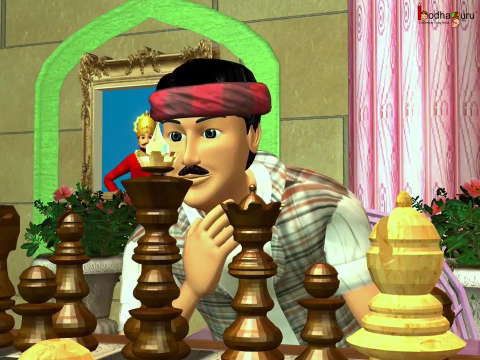 This is so good. I am very happy. Tell me what kind of reward you deserve for this great invention. If you think this is invaluable, then just give me half of the treasure of the kingdom. Don't you think that is asking for too much? 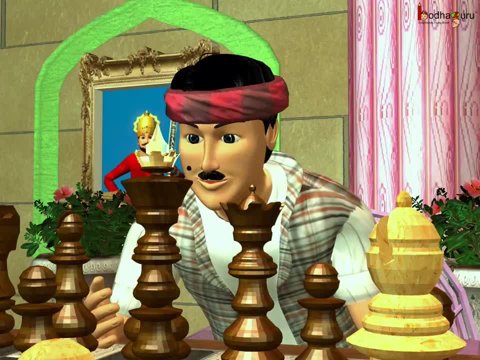 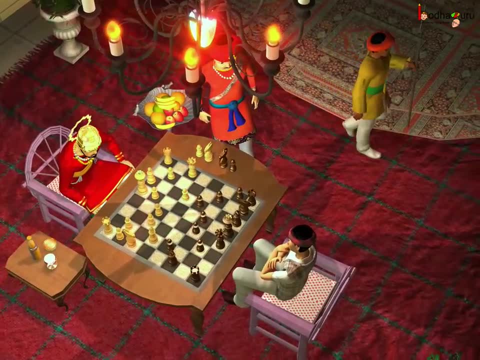 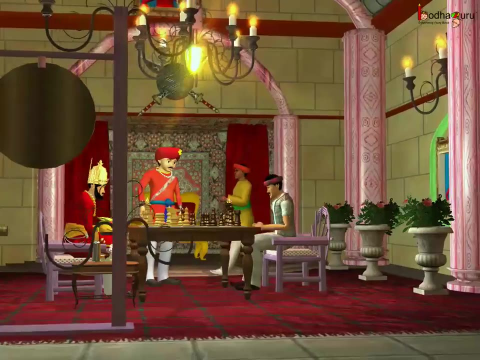 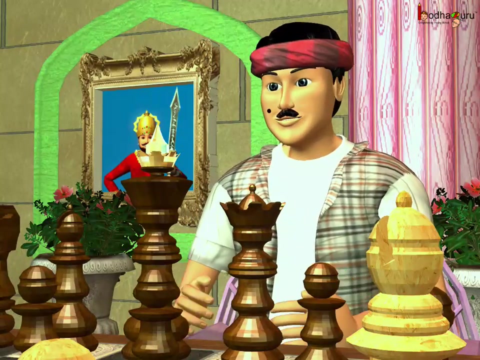 I am so sorry, your majesty, I became little greedy. Say: how about? for the first square of the chessboard, I receive one grain of wheat, two grains of wheat, for the second, Four, for the third one and so forth, doubling the amount of grain each time. 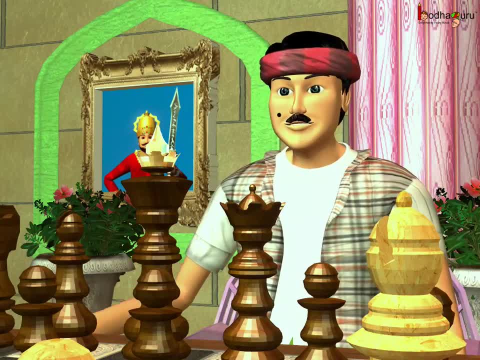 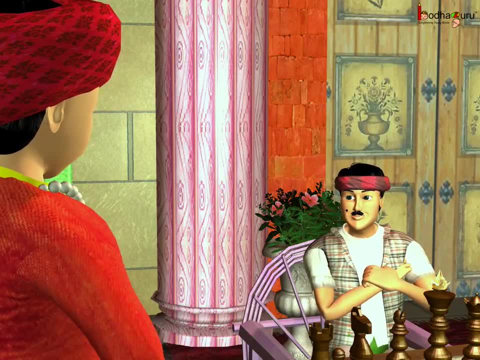 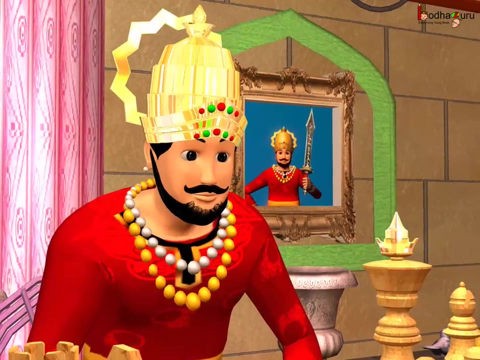 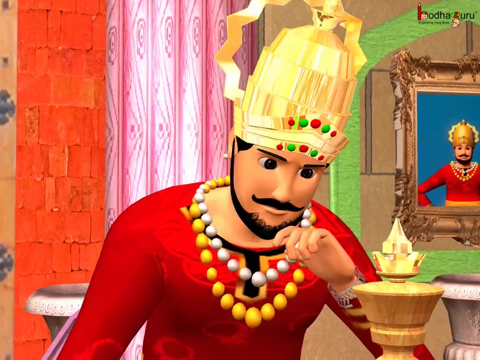 There are just 64 squares on the board. It is not asking for too much, is it wise, minister? Now is he making fun of me by asking for so little. Anyways, if he wishes for so less, let him have it. 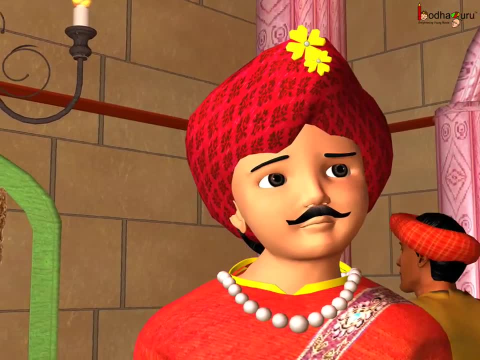 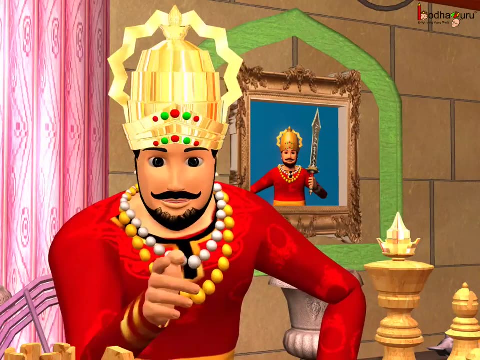 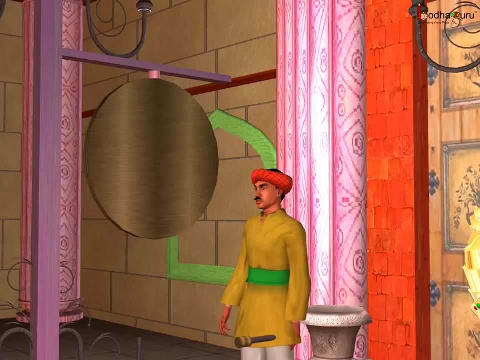 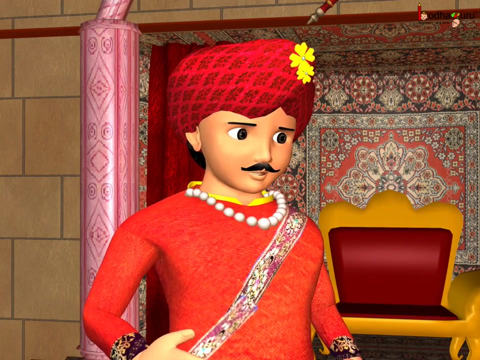 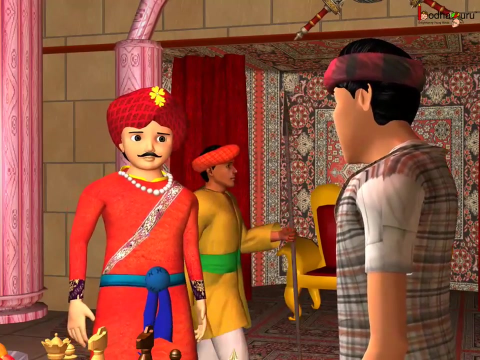 Hmm, something is fishy here, I know for sure this man is too greedy. Agreed, But on one condition: It's time for king to take rest. What Our lord will take rest now. let us meet tomorrow. Whatever you say, I accept. wise minister, thank you, my majesty. 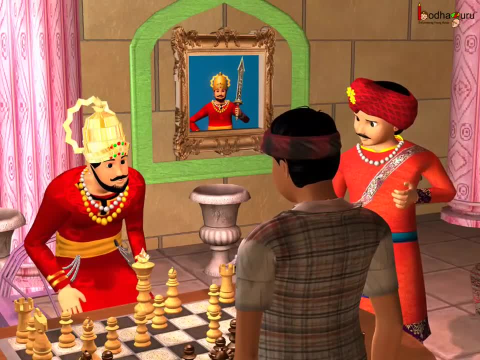 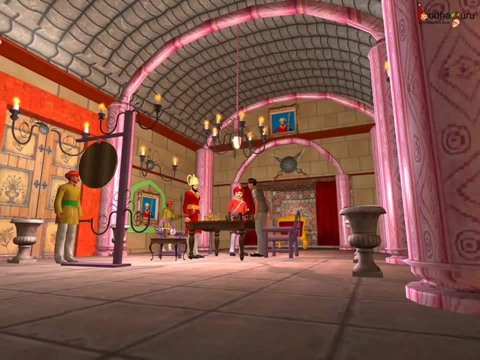 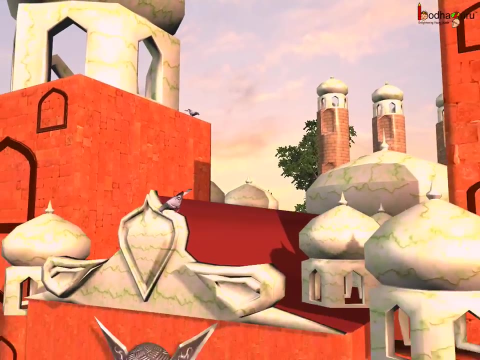 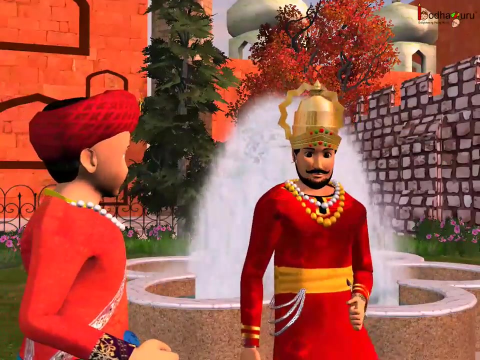 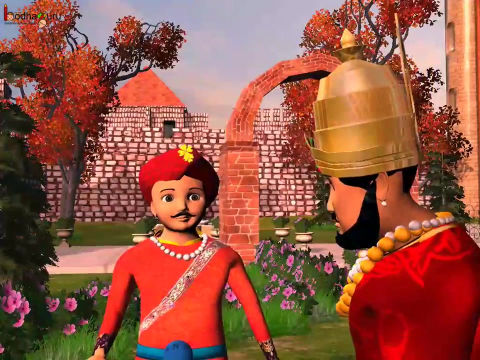 As you say, my wise minister. so let us meet tomorrow. I will be back, I will be back. Why didn't you give him what he asked for and finished his request right away? Anyway, he had asked for so little, My lord. what he asked for was: 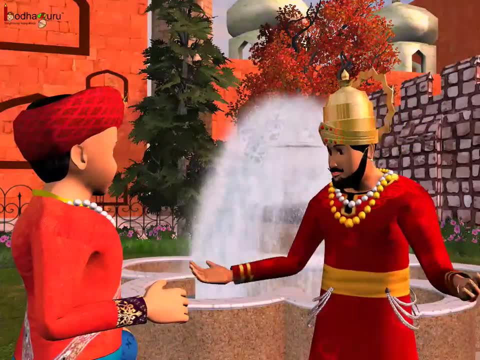 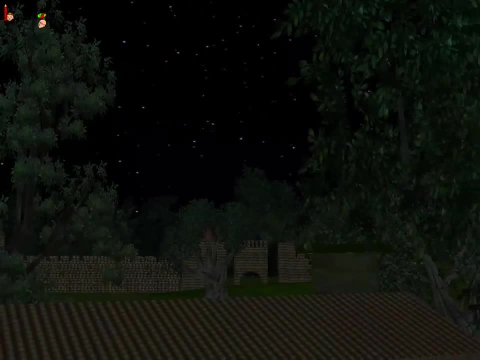 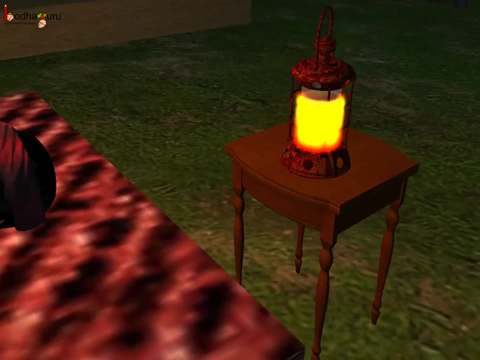 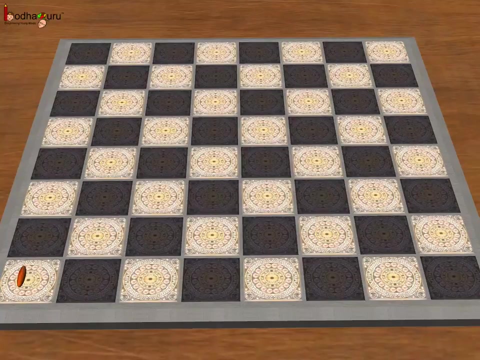 Oh really, I never saw this way. I never saw this way. There he is. there. he is my lord. Is this what you have been looking for? The throne of the king has been served. Let me have a look at the other things he has brought. 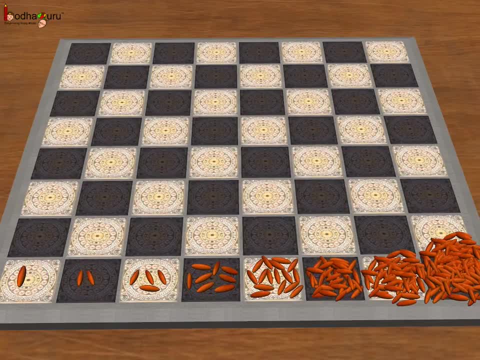 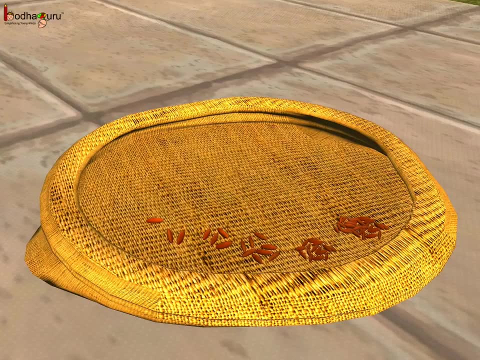 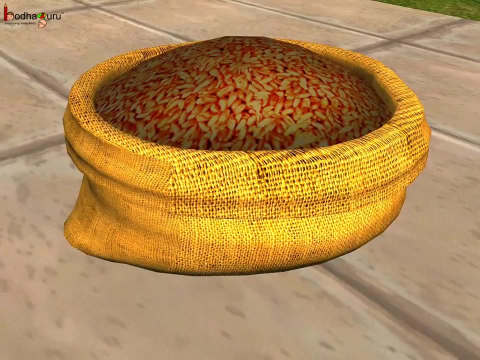 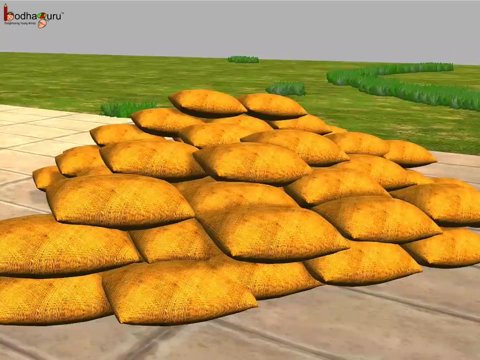 Oh, there he is, my lord, my king. Well, I hope it's him. Let us meet him tomorrow, wise minister, So that we may meet again. Oh, look at him again. Oh, good to see you. Slowly, one bag after another is getting filled. the minister is getting tired, the entire. 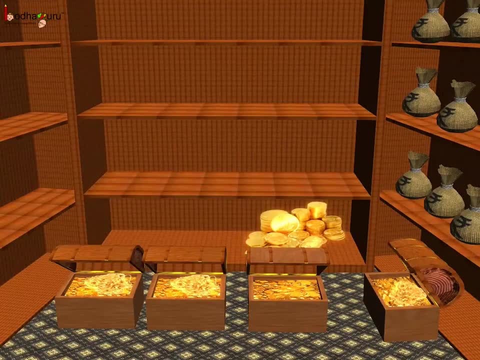 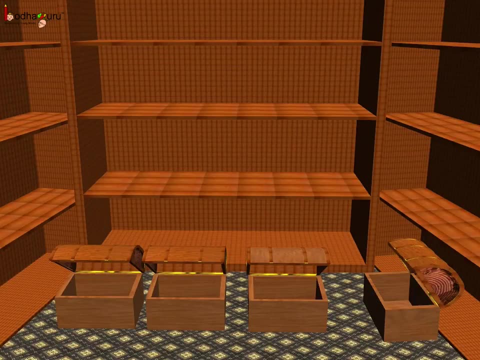 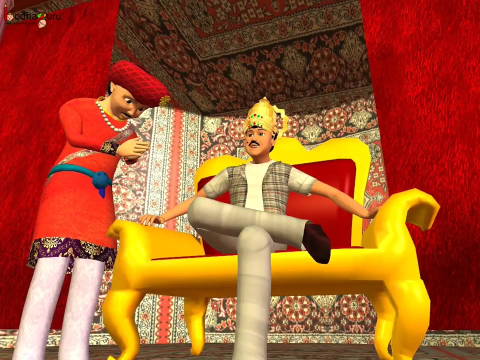 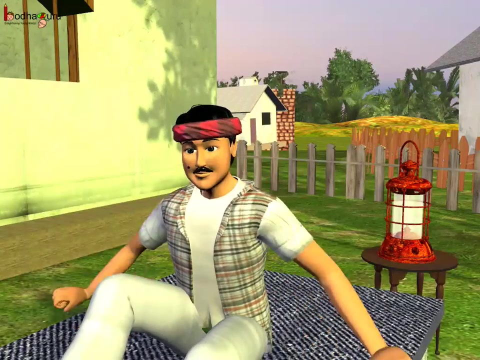 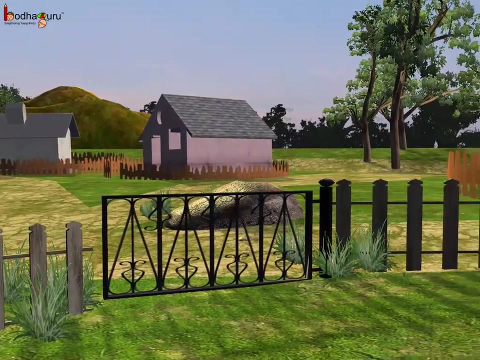 kingdom treasure is getting empty as the king is buying grains from the sellers. Finally, the king's treasure is left with nothing. the king gave his crown to the man and he became the king himself. oh, that was such a nice dream. early morning dreams are. 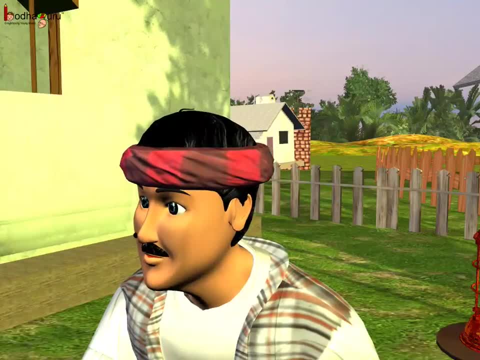 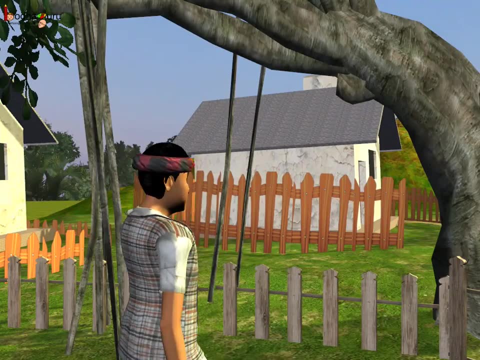 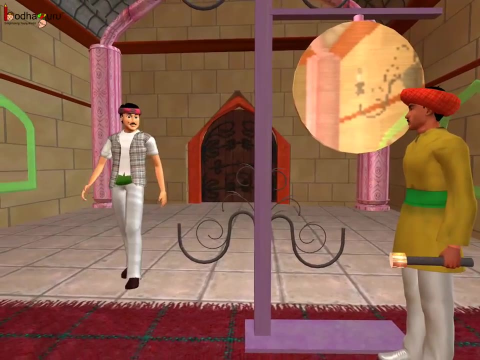 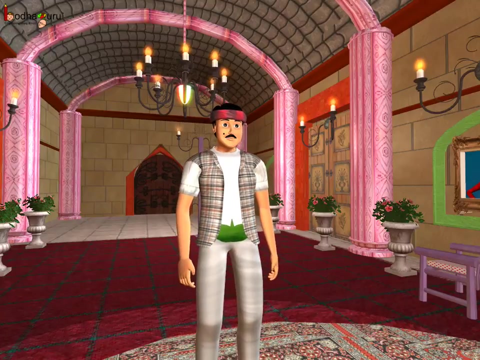 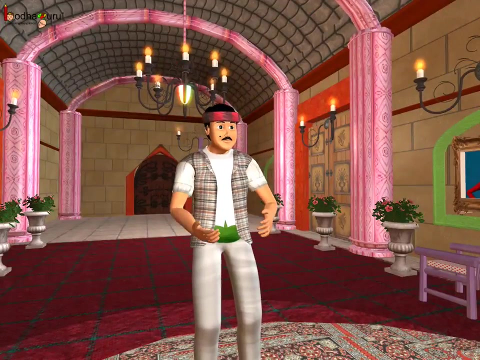 always true. Today, I shall be crowned as king. Let me get ready fast. Your majesty, I am ready to collect my reward. What is your condition, vice minister? What is your condition, vice minister? What is your condition, minister? 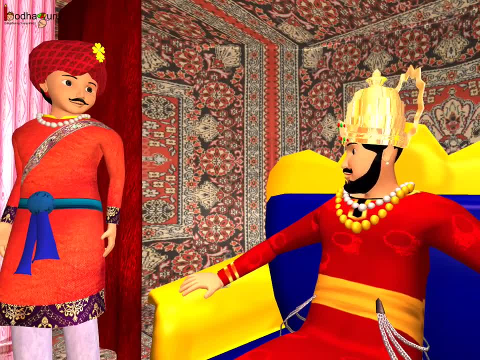 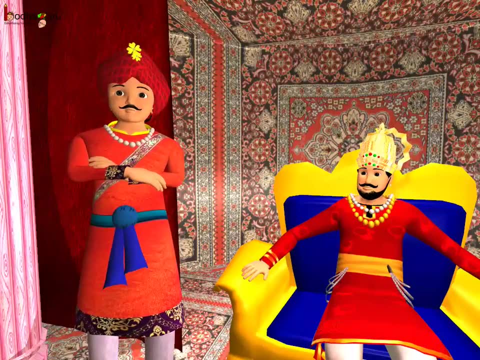 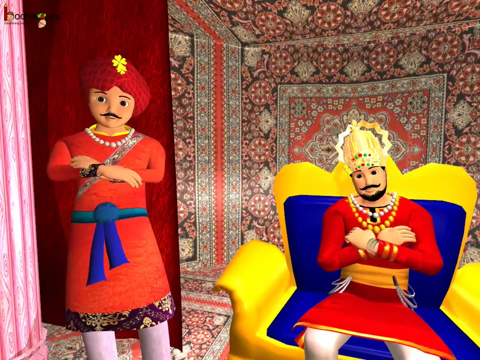 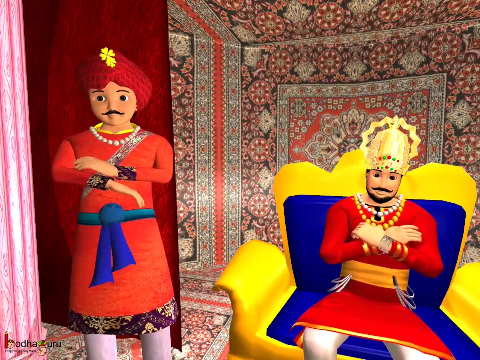 Nothing much. as promised, you shall receive one grain of wheat for the first square, two for the second one, four on the third one, and so forth, doubling the amount each time for the sixty four squares of the chess board. Today, I will become king.